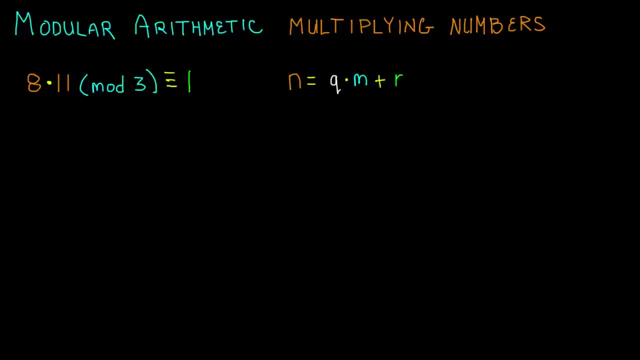 Hey everybody, this is Paul. In this video I'm going to be explaining how to multiply two numbers together when we're dealing with modular arithmetic. So here I've got 8 times 11 in mod 3 is congruent to 1.. So the way we get this solution is by using this formula right here, where you take the original number- in this case, the original number is 8 times 11 or 88, and then we place the mod number here- in our case that would be 3 here- and then we just fill in the q and r as the original number. 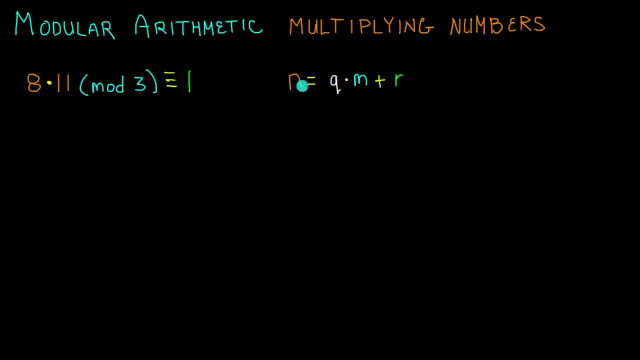 As needed to make this a true statement. And when this is a true statement, then we can say that this number n over here- or in our case it will be 8 times 11, we can say that that's congruent to the remainder. So let's go ahead and do that, and I'll show you a couple different ways that we can go ahead and do this. So let's just go ahead and multiply 8 times 11 and that gives us the value 88.. So we'll go ahead and write 88 down And we're just going to use this equation here and fill in q and r as needed to make this a true statement. So we have: 88 is equal to. 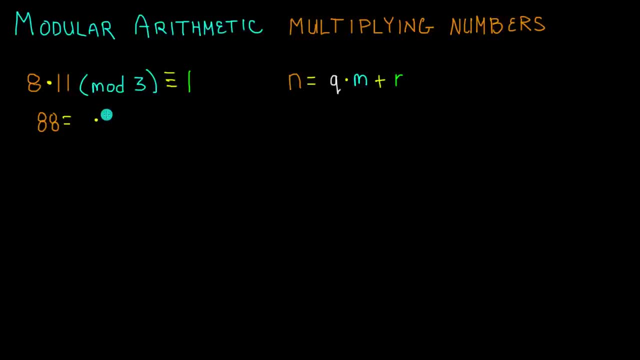 some number q times our mod, which is 3, plus some remainder. So since 88 is a positive number, we want to pick a q so that q times 3 is the biggest number possible without being bigger than 88. So it turns out that 29 times 3 will give us the value 87,, which is the biggest integer we can choose for q and still have that value less than 88. So let's go ahead and write 29 down here. 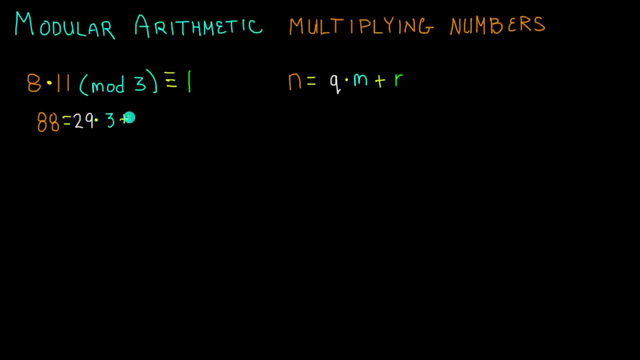 so 88 is equal to 29 times 3 plus some remainder. so 29 times 3 is 87. so then 87 plus 1 is equal to 88, and so the reason why I'm calling this 1 or remainder here is because, if we think about this, 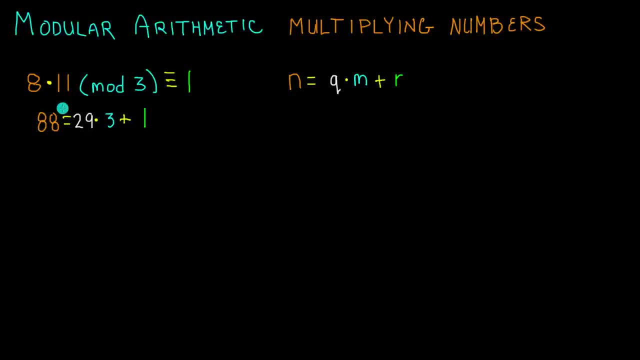 we take the number 88 and we divide it by our mod. so 88 divided by 3 is equal to 29 plus the remainder of 1. so now we've got it in this form of n is equal to qm plus r, and once we get it there, 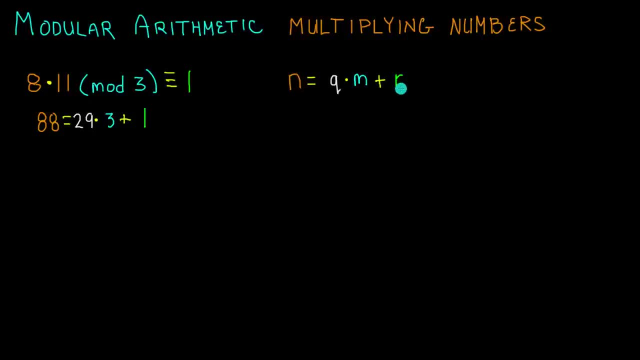 we can just say that n, the number we started with, is congruent to our remainder when we're dealing with that mod. so in our case, 88 is congruent to 1 when we're dealing with mod 3, which is what we have right here. so that's one way to solve this problem. let's go ahead and look at: 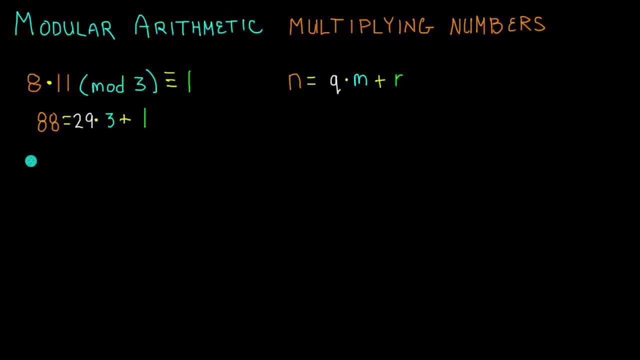 another way. so let's look at this 8 right here, and we'll go ahead and write it like this. we'll go ahead and put it in some brackets here, and the brackets are just a grouping mechanism. putting this in brackets won't change its value at all, and so let's write this as 8 mod 3 and then we'll close. 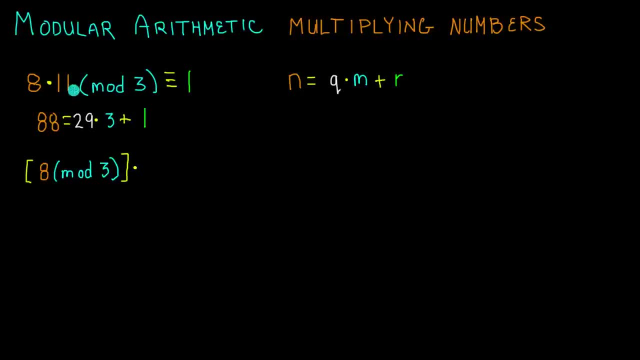 the box and we'll go ahead and write it like this, and we'll go ahead and put it in some brackets here, and then that's multiplied by the 11, so we'll put the 11 in brackets as well, and we'll write 11 as 11 mod 3. so, for this example, what i want to do is i want to show you that you can. 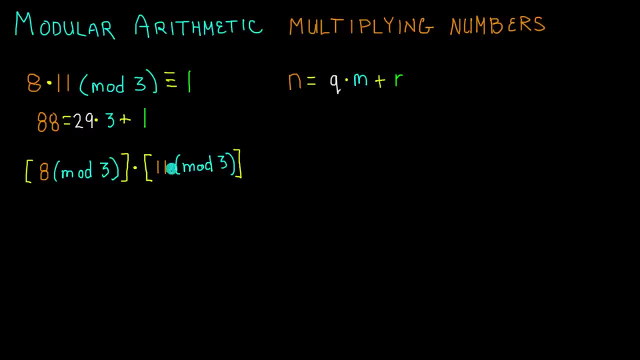 first convert 8 and also convert 11 and then take the results from each of those. multiply those results together and you'll still find the solution that you're looking for. if we want to find 8 mod 3, we'll just plug it into this equation here. so our n is the number we're starting with. 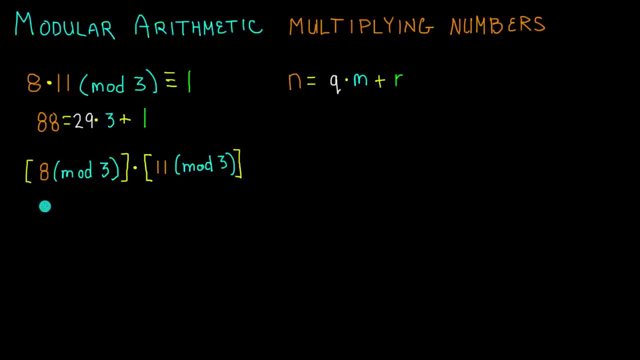 we're starting with 8. we want to know what 8 is congruent to in mod 3. so our n is 8, and then that is equal to some q value multiplied by m, and m is our mod. so that's 3 plus some remainder. so we want to pick the largest value of q, so that q times 3 is as. 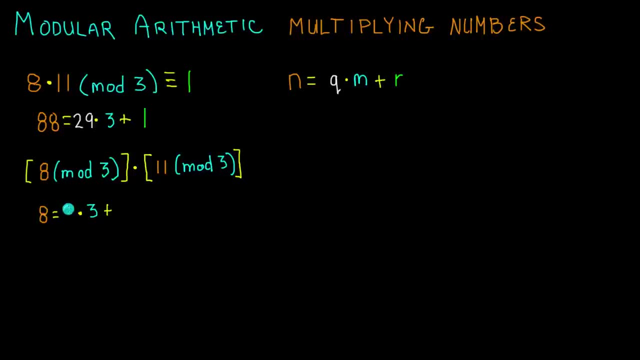 big as possible, but less than 8. so we're going to pick a q value of 2, since 2 times 3 is 6 and that's the biggest q we can use to make q times 3, still less than 8. so we have: 8 is equal to 6. 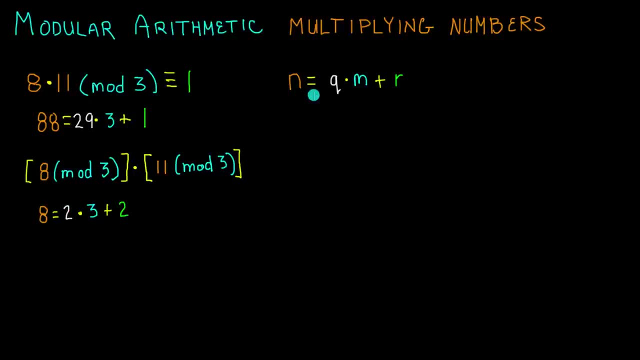 and then we'll have a remainder of 2. so now we've written this in this: n is equal to q, m plus r form again, so that tells us that 8 is congruent to the remainder. we can rewrite 8 now as the value 2, so i'll just put a 2 here now. let's do the same. 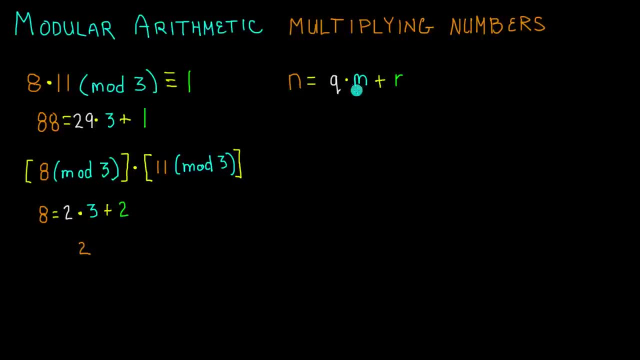 thing for 11 mod 3. so plugging this into n is equal to q, m plus r. n is what we're starting with. that's the 11, and n is equal to some q multiplied by our mod of 3 plus some remainder. once again. 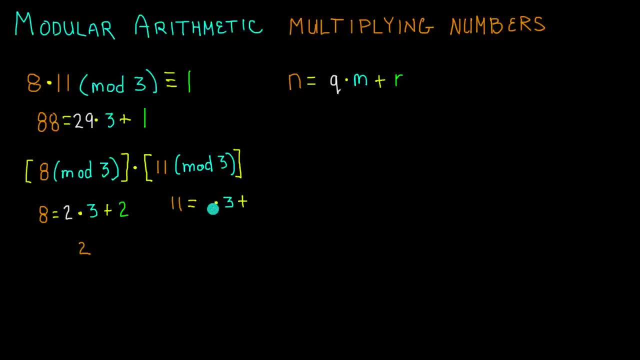 since 11 is a positive value, we want to pick the q so that q times 3 is as big as possible. and then we continue with: n is equal to passive n, and we'll look at 5 to get proof that Q is 2, and then we can put a matching Q here with Q value. we'll do that in a second, and then we'll repeat 11. so we have f or some other value here. so for nine plus two is equal to 11. so no, we have this in. the. n is equal to Q, m plus r form, and so now that we've. 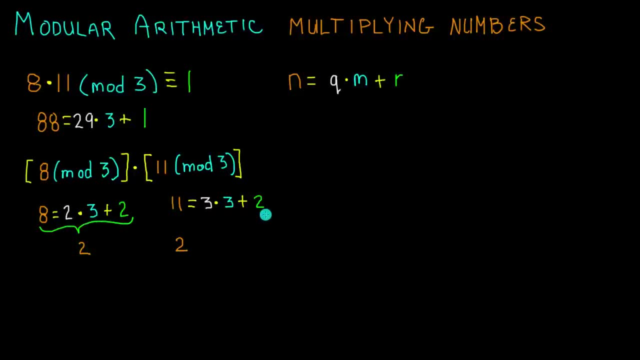 created this AND, and so now we've made confession of q. thank you strong. so now that we've created a true statement here, we can say that 11 is congruent to our remainder of 2 when we're dealing with mod 3 to 2- mod 3, and we also found that 11 is congruent to 2- mod 3. so we've simplified this a little bit. 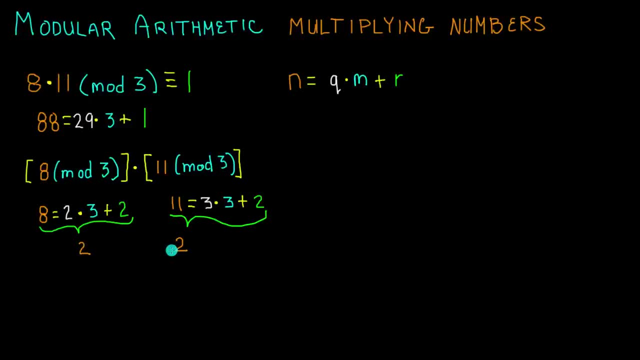 so instead of 8 times 11, we can now write 2 times 2 mod 3. so let's go ahead and do that. so we'll just go ahead and move these over to the other side of the screen here. so now we have this new. 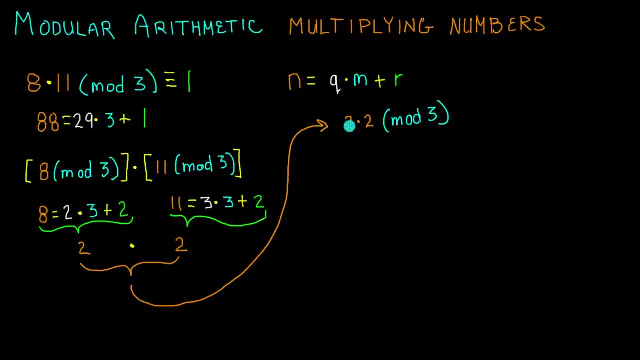 problem: 2 times 2 mod 3. so now what we can do is we can say: 2 times 2 is equal to 4, and so now we're looking at 4 mod 3 and then once again, we can just simply plug this into our: n is equal to. 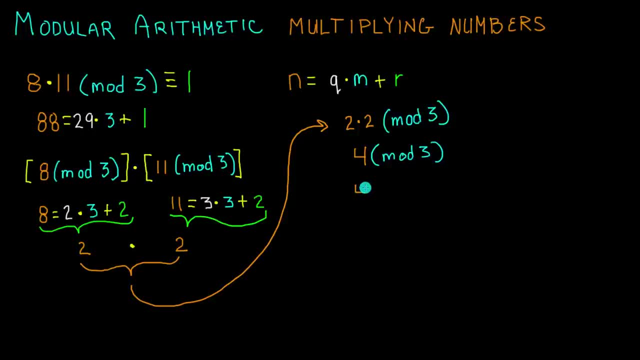 qm plus r. so n is the number we're starting with. we're starting with the value 4, and that's equal to q times m, and m is our mod, which is 3, and that's plus some remainder. so once again we want to find the q so that q times 3 is as big as possible, but less than 4. so in this case q is. 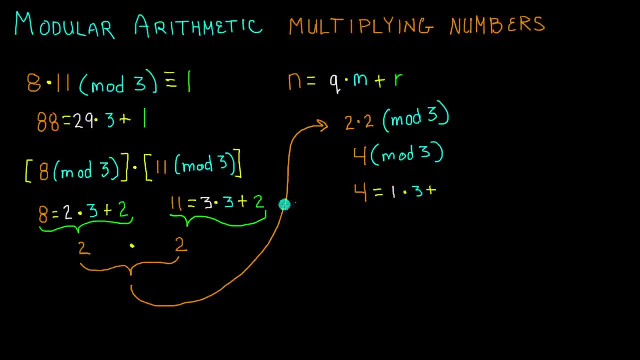 going to be 1. 1 times 3 is 3, and then we add a remainder of 1, and so this should be equal to the value of q, and this should be equal to the value of m, so we can add a remainder of 1, and so this should be equal to the number of mod 3, and then we 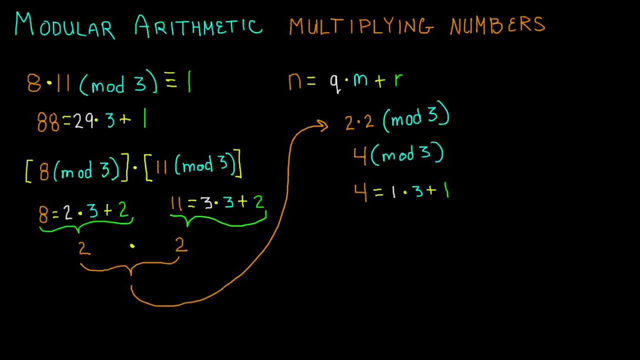 us here that 4 is congruent to 1 mod 3.. So we'll go ahead and write that down: 4 is congruent to 1 mod 3.. So what I illustrated here is: I just wanted to show you that there's more. 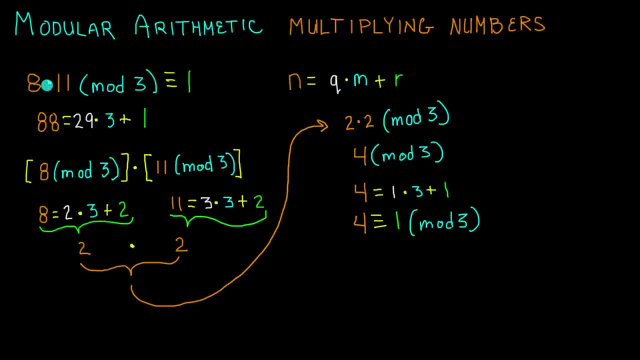 than one way to do this. We could have either just said: okay, 8 times 11 is 88. I'm going to plug that into this equation and then from that I can see that 88 is congruent to the remainder of 1 mod 3.. The other thing we could do is we could say: 8 times 11 mod 3 is the. 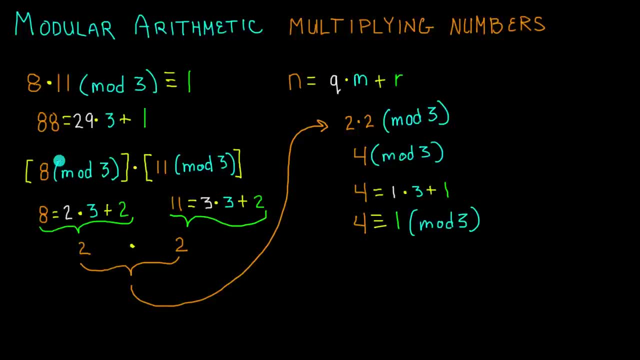 same thing as 8 mod 3 times 11 mod 3.. And then we can figure out what 8 is congruent to in mod 3 by plugging it into this equation here, And we can do the same thing with 11.. 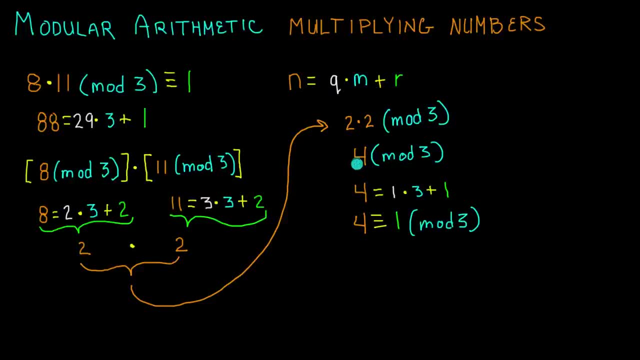 So that gives us the new equation of 2 times 2, or 4 mod 3. We can plug 4 into this equation and we can find that 4 is congruent to 1 mod 3. And by finding this relationship we can: